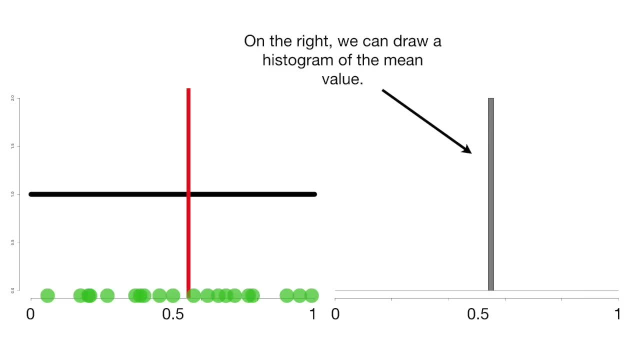 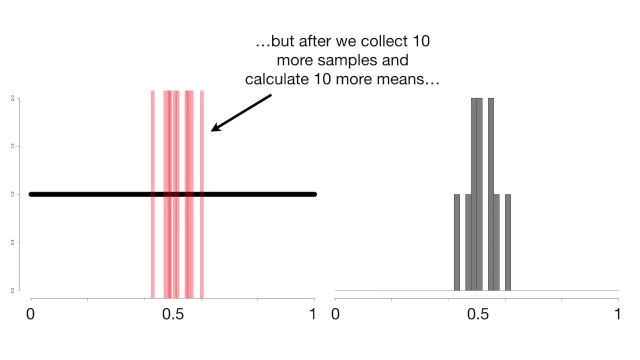 calculate the mean of the samples And on the right we can draw a histogram of the mean value. Since we only have one mean value, the histogram isn't very interesting. But after we collect 10 more samples, and collect 10 more means the 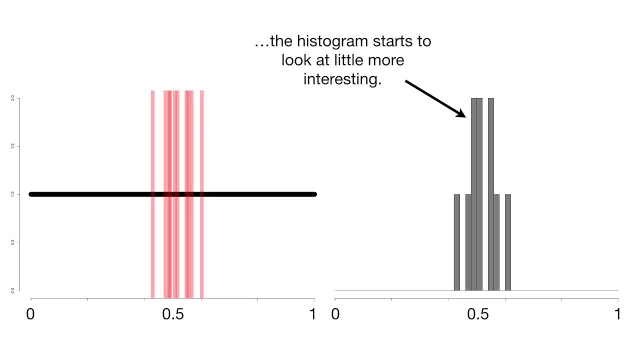 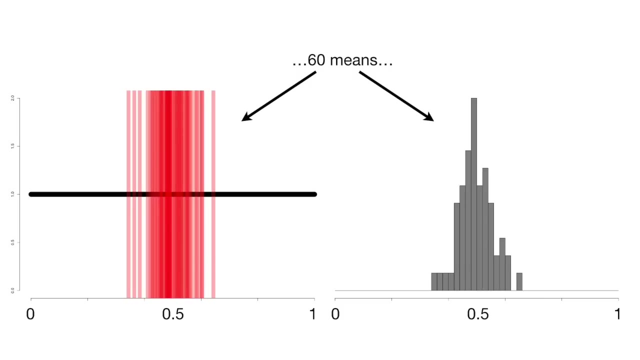 histogram starts to look a little more interesting. Here's the Histogram: after collecting 20 samples and calculating, 20 means, 30 means, 40 means, 50 means, 60 means, 70 means, 80 means, 90 means and 100 Means. After adding 100 means to the: 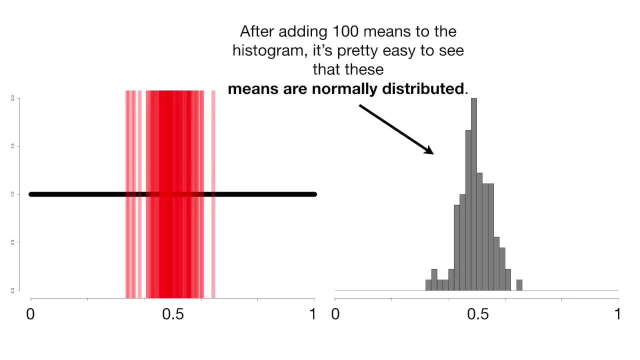 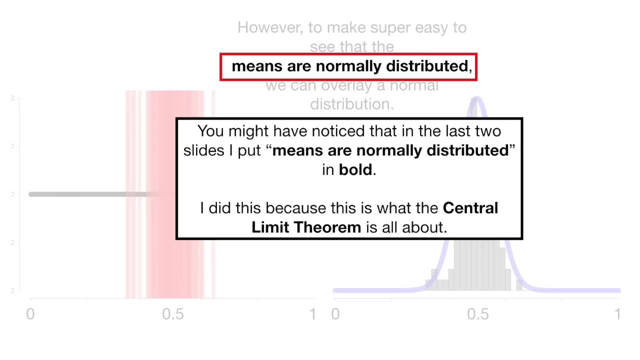 histogram. it's pretty easy to see that these means are normally distributed. However, to make it easy to see that the means are normally distributed, we can overlay a normal distribution. You might have noticed that in the last two slides I put means are normally distributed in bold. 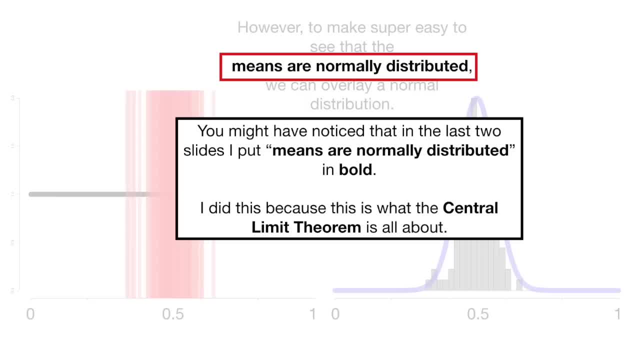 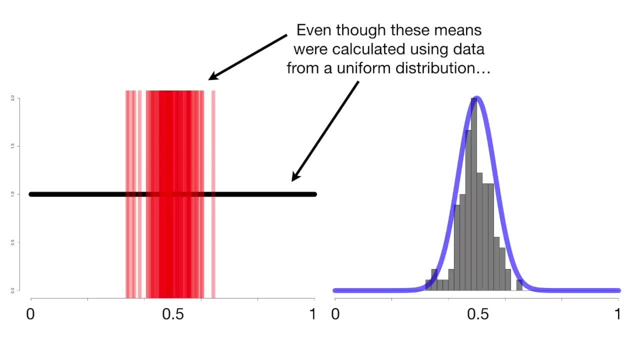 I did this because this is what the central limit theorem is all about. Even though these means were calculated using data from a uniform distribution, the means themselves are not uniformly distributed. Instead, the means are normally distributed Bam. Here's another example. 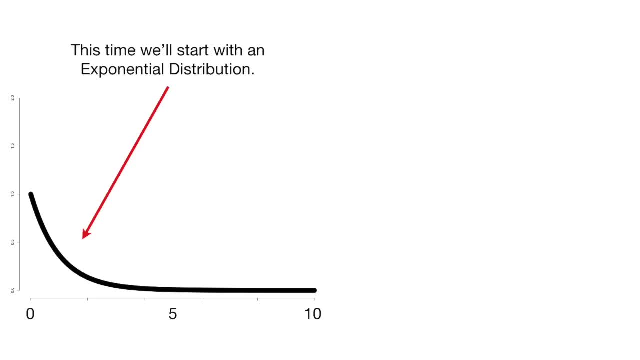 This time we'll start with an exponential distribution. Just like before, we can collect 20 random samples from this exponential distribution And, just like before, we can calculate the mean of the 20 samples. And, lastly, we can draw a histogram of that mean over here on the right. 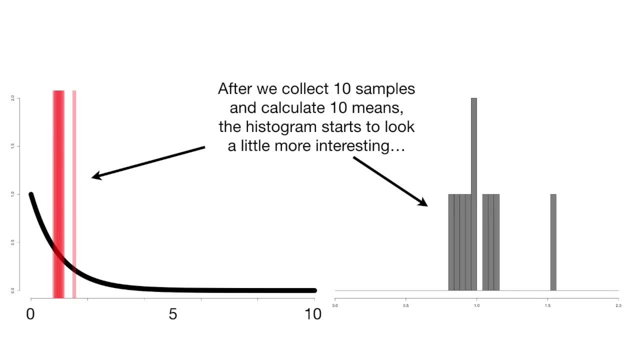 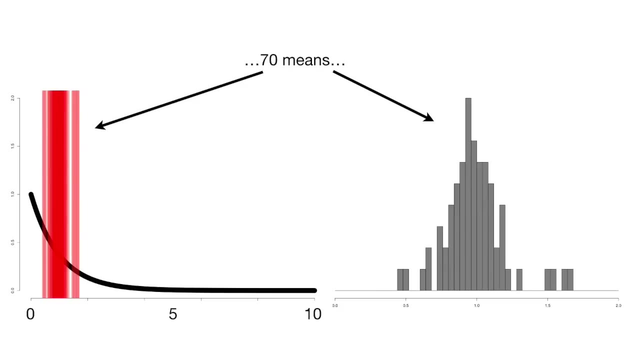 After we collect 10 samples and calculate 10 means, the histogram starts to look a little more interesting. Here's the histogram after: 20 means, 30 means, 40 means, 50 means, 60 means, 70 means, 80 means, 90 means and 100 means. 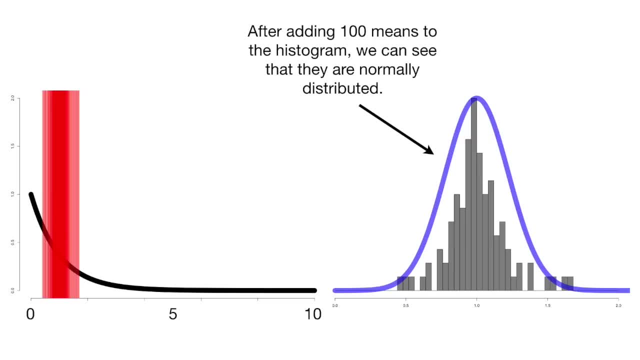 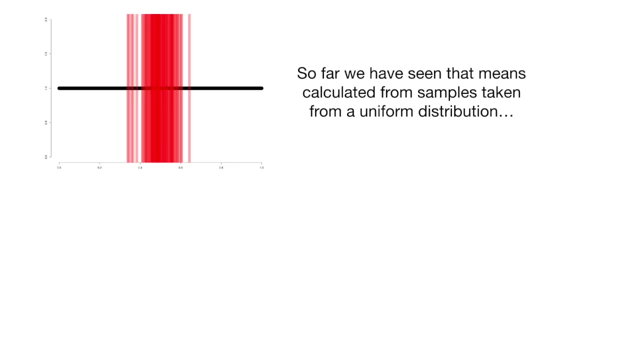 After adding 100 means to the histogram, we can see that they are normally distributed. Even though these means were calculated using data from an exponential distribution, the means themselves are not exponentially distributed. Instead, the means are normally distributed. Bam So far, we have seen that the means calculated from samples 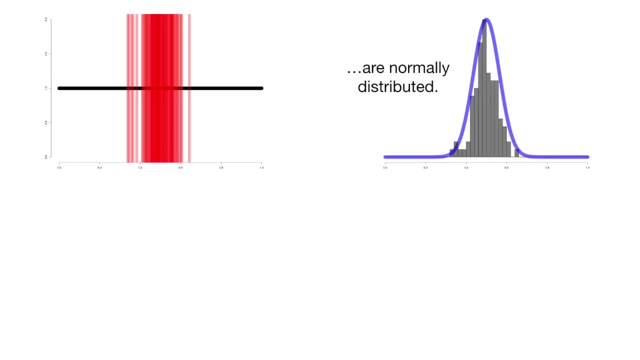 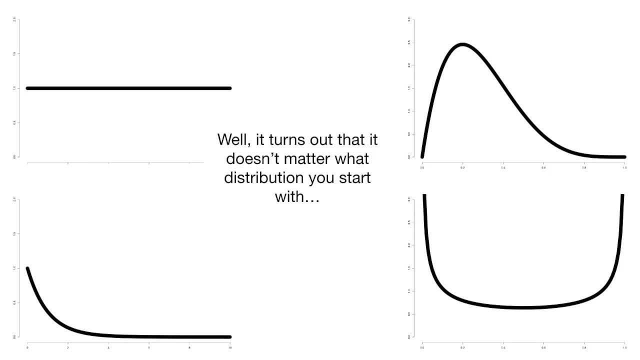 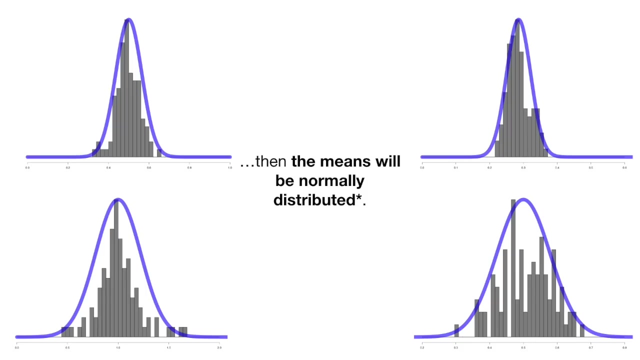 taken from a uniform distribution are normally distributed, and means calculated from samples taken from an exponential distribution are also normally distributed. Well, it turns out that it doesn't matter what distribution you start with. If you collect samples from those distributions, the means will be normally distributed. 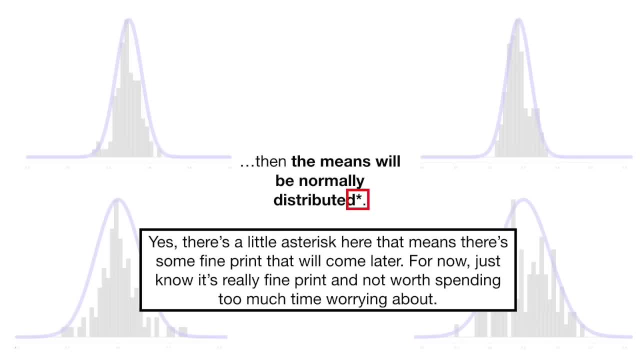 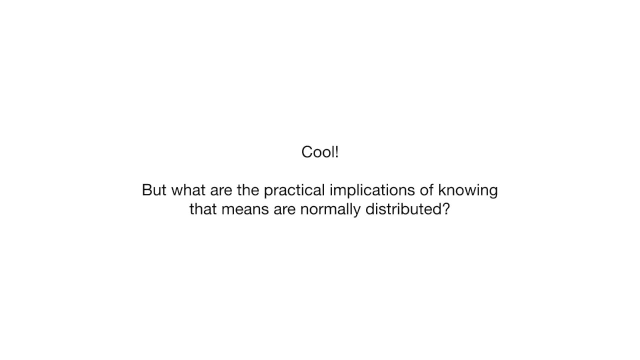 Yes, there's a little asterisk here. that means there's some fine print that will come later. For now, just know it's really fine print and not worth spending too much time worrying about Double bam Cool. But what are the practical implications of knowing that the means are normally distributed? 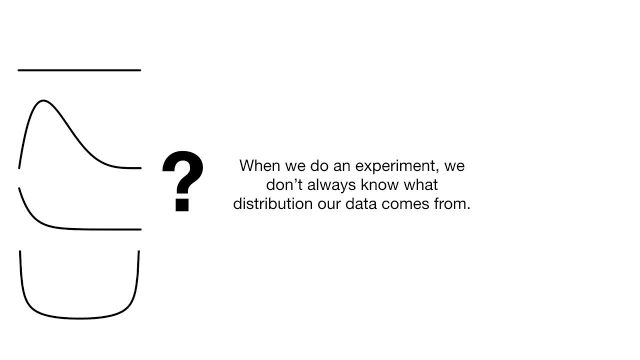 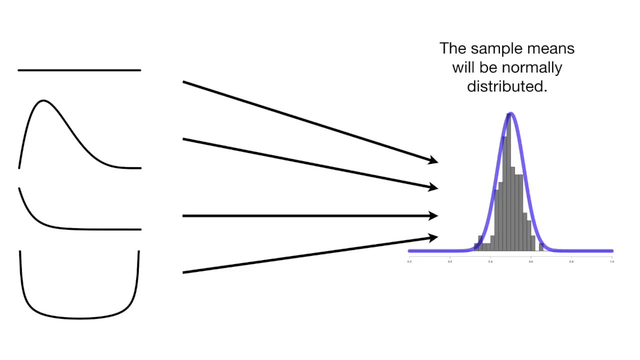 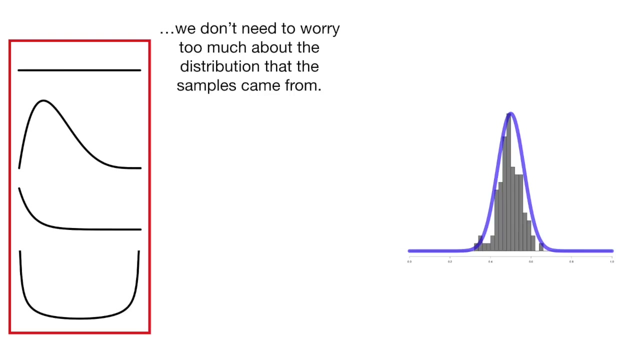 When we do an experiment, we don't always know what distribution our data comes from. To this, the central limit theorem says: who cares? The sample means will be normally distributed. Because we know that the sample means are normally distributed, we don't need to worry too much about the distribution that the samples came from. 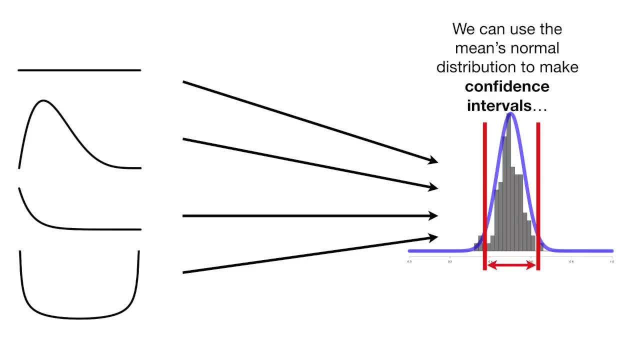 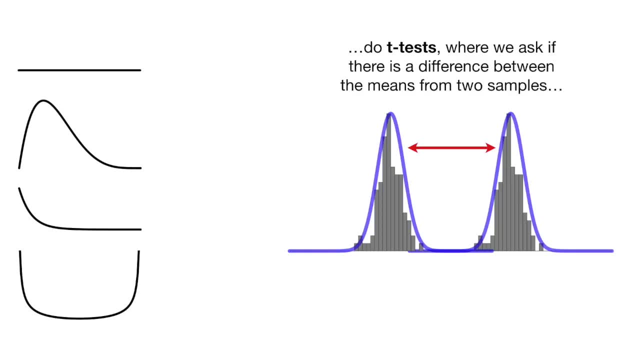 We can use the means normal distribution to make confidence intervals, do t-tests, where we ask if there's a difference between the means from two samples, and ANOVA, where we ask if there is a difference among the means from three or more samples, and pretty much any statistical test that uses the sample mean. 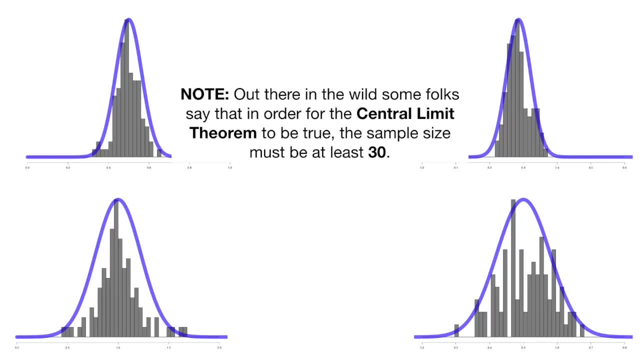 Triple bam Out there in the wild. some folks say that in order for the central limit theorem to be true, the sample size must be at least 30. This is just a rule of thumb and generally considered safe. However, as you can see in the examples here where I use a sample size of 20,,